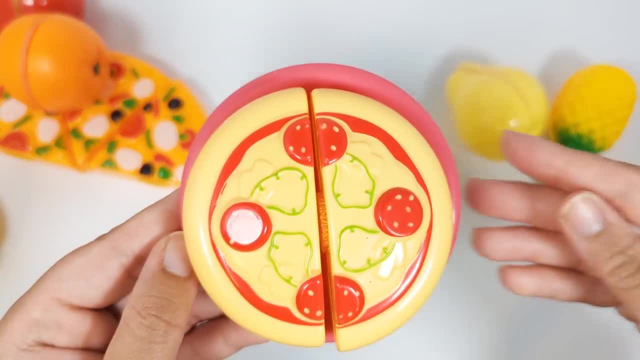 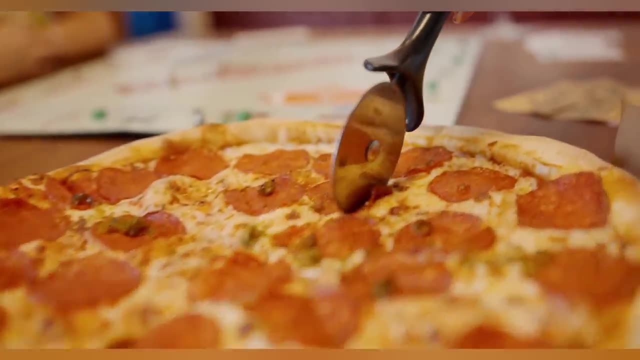 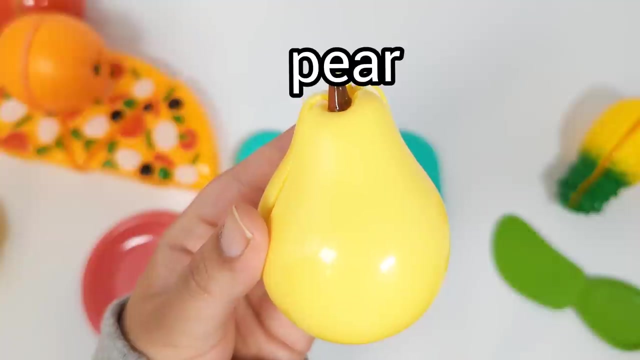 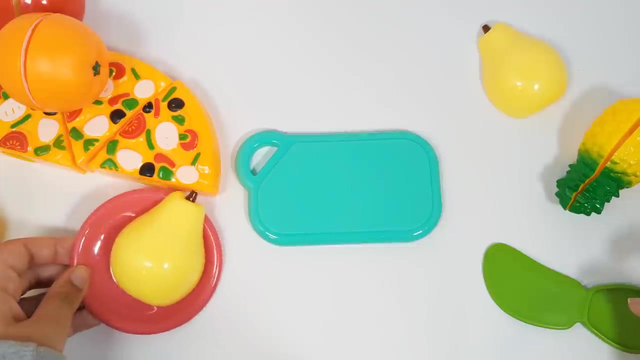 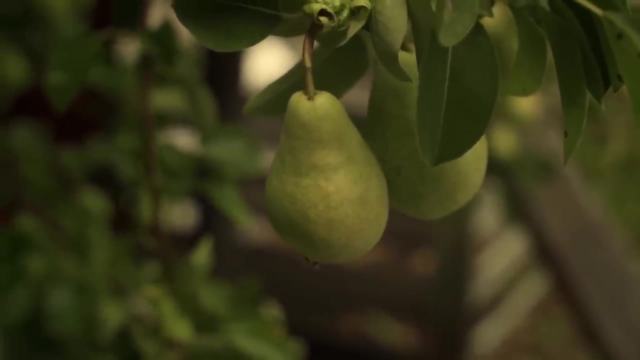 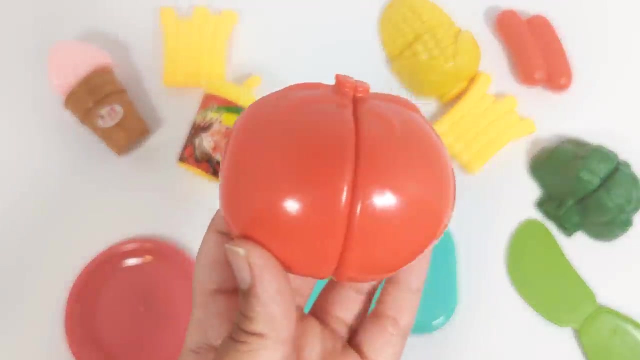 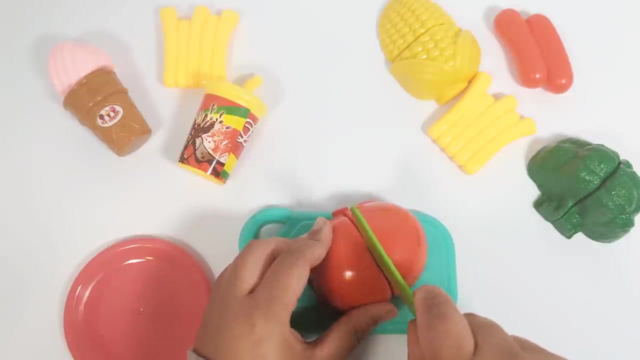 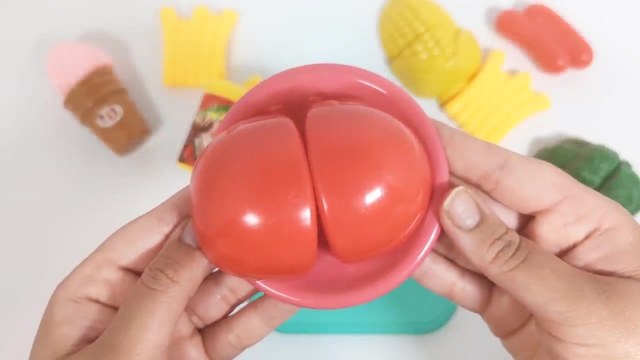 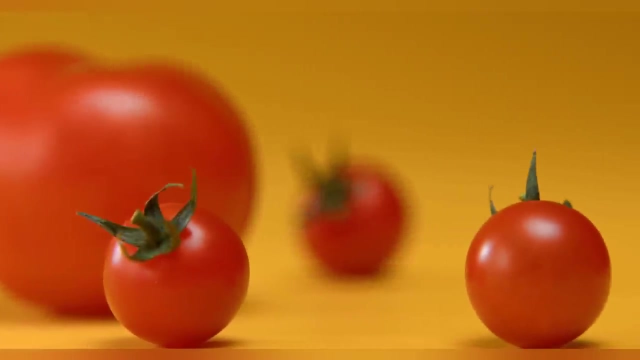 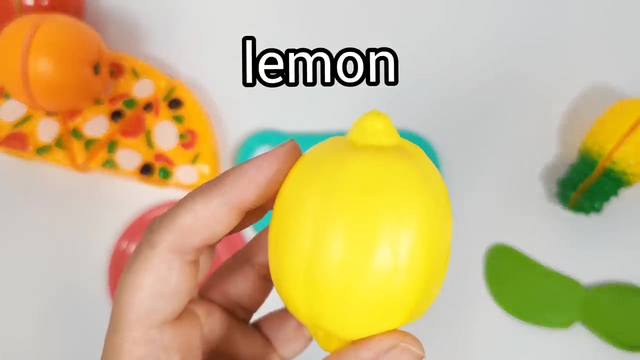 Pizza. This is a pear. A pear is a delicious fruit. Oh, it's a pear. Oh, it's a pear Pear. This is a tomato. A tomato is a red fruit Tomato. This is a lemon. Lemons are really sour. 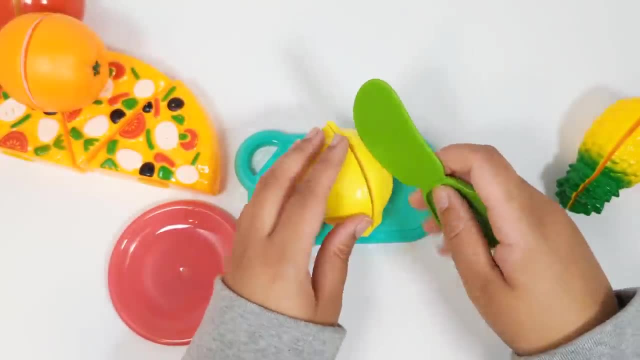 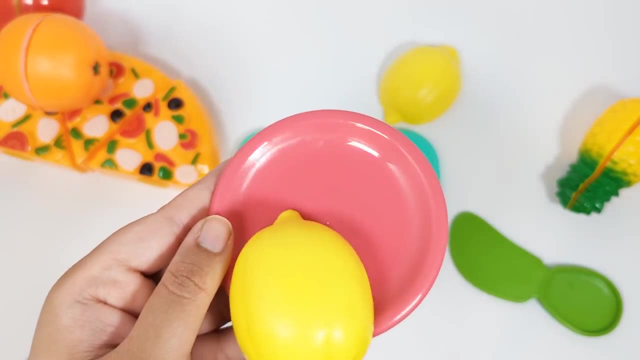 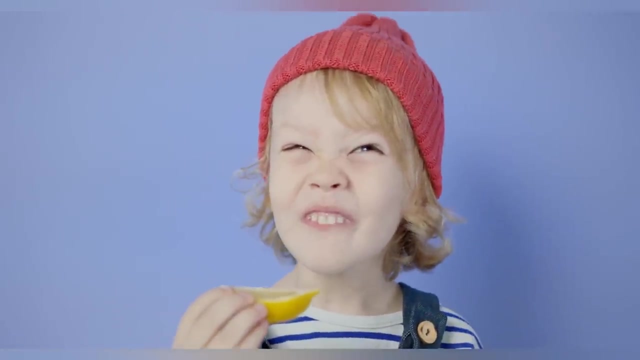 It is also a fruit: Lemon, Lemon, Lemon. This is a green apple. Lemon, Lemon, Lemon. This is aTHIS IS A SPOON. This is a mango. I don't know what this is, though- A banana. 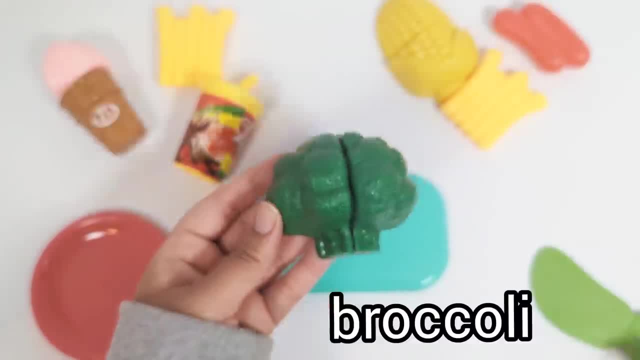 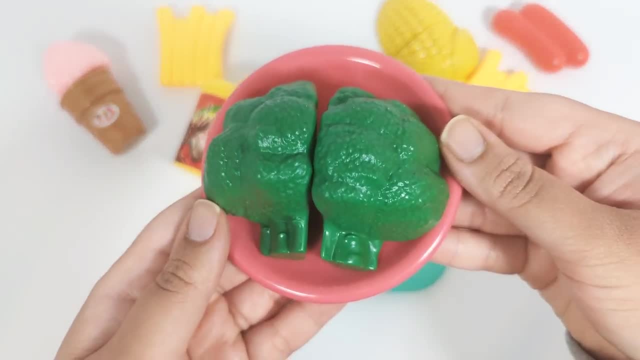 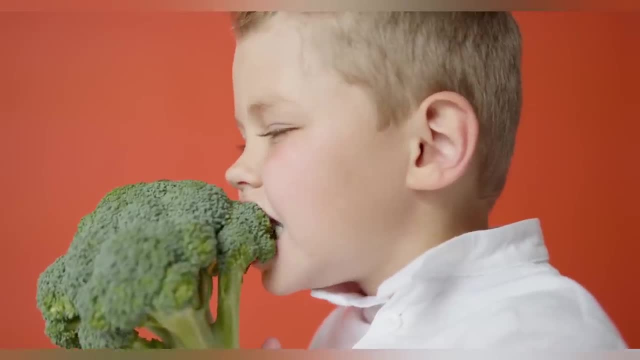 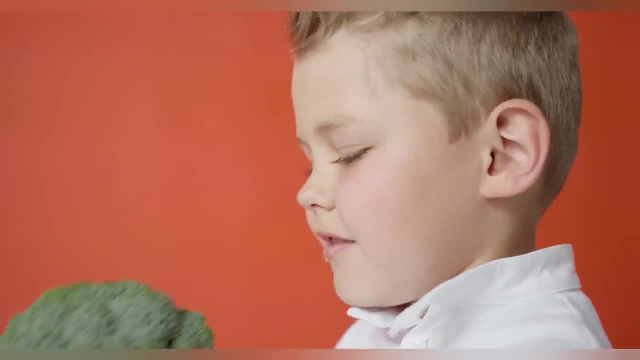 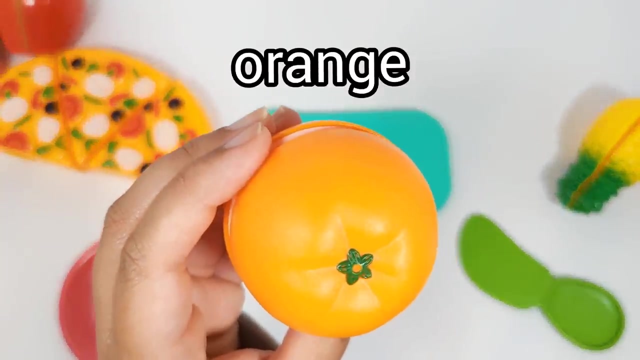 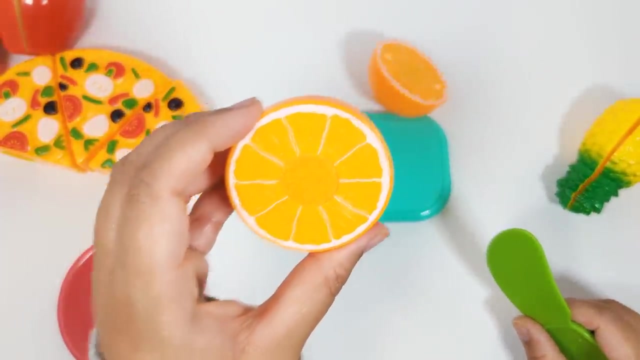 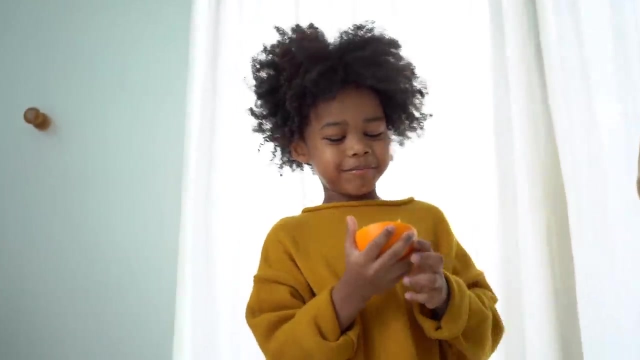 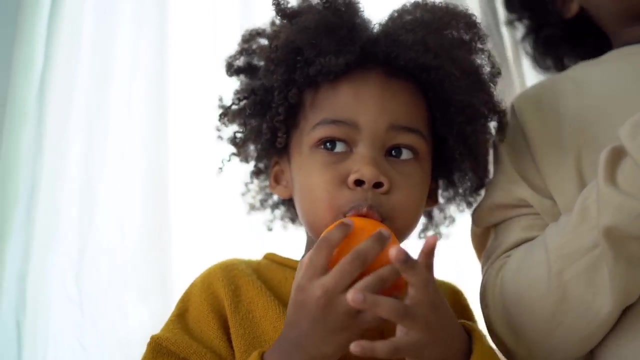 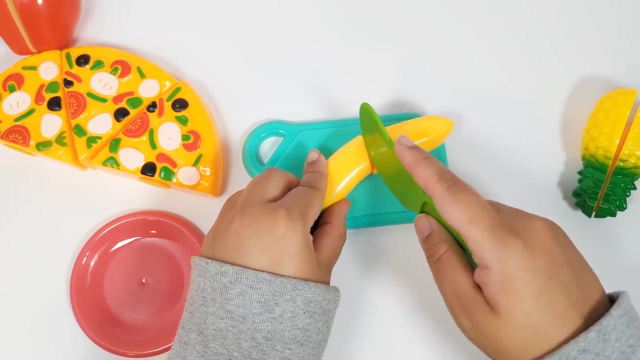 I'll give you another. OK, Thank you, Thank you, OK. Okay, This is an orange. An orange is a yummy, delicious and juicy fruit. This is an orange. This is a banana. A banana is a very healthy fruit. 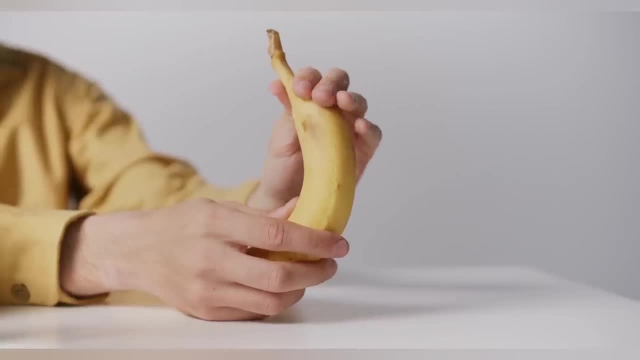 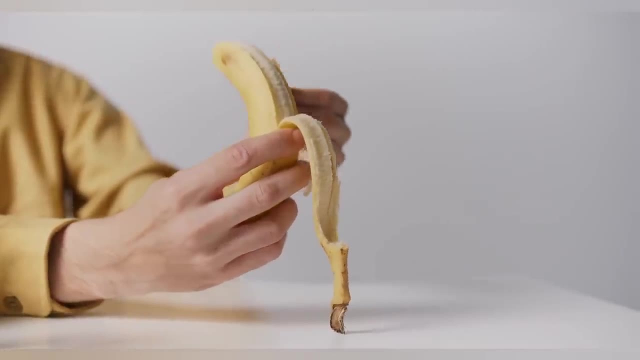 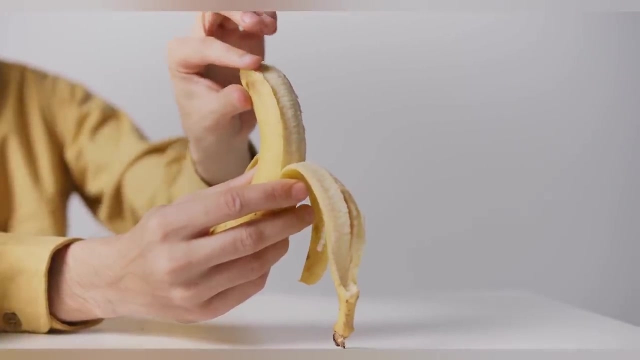 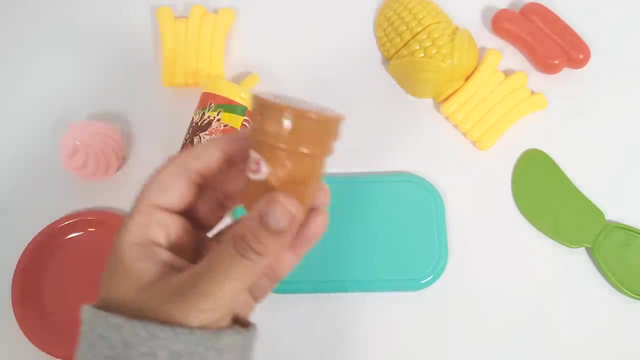 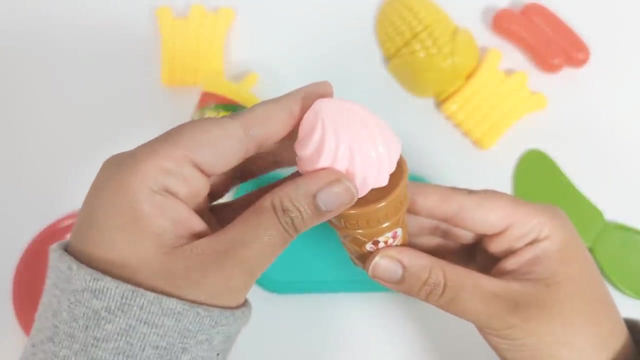 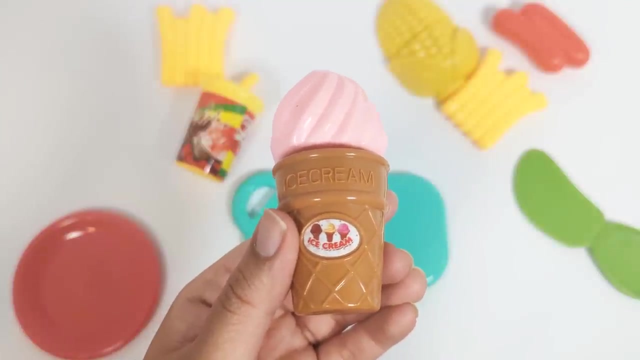 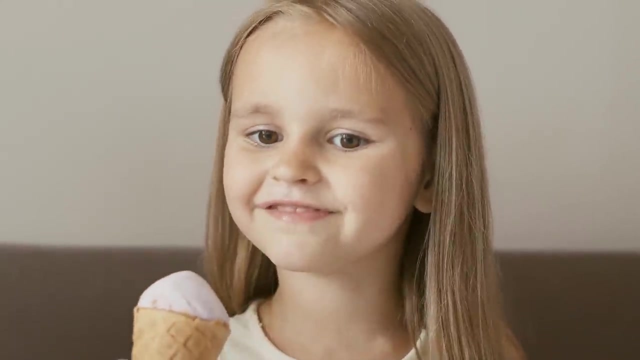 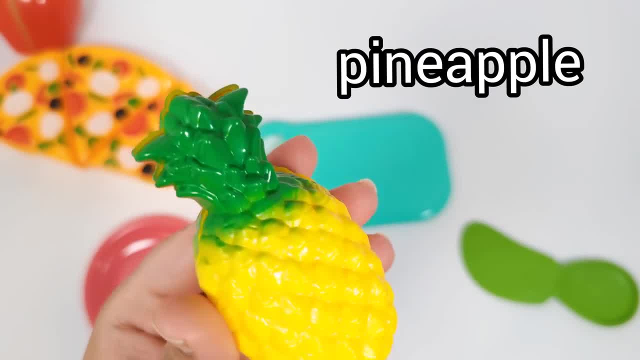 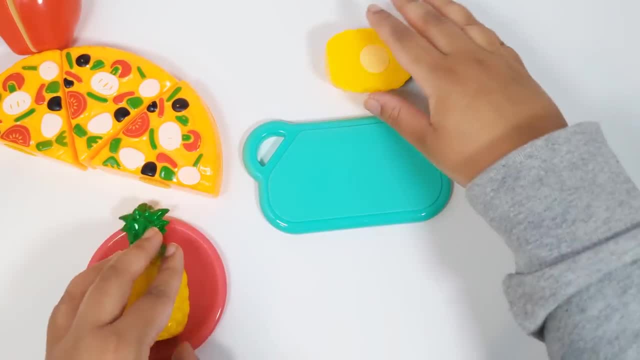 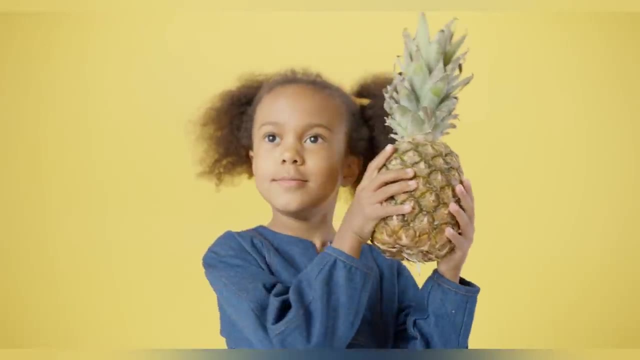 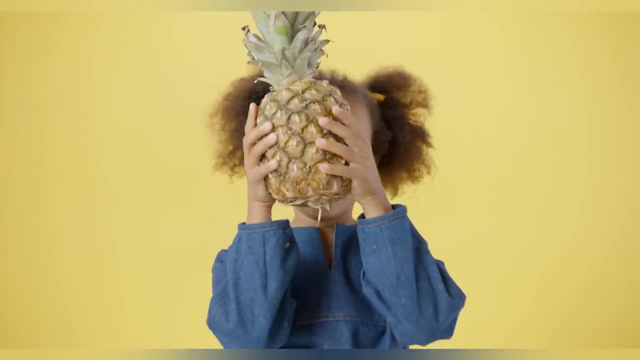 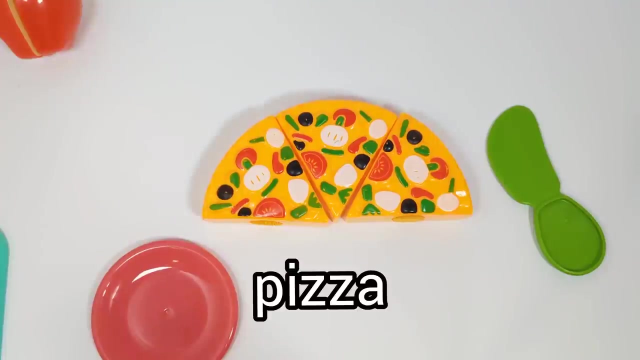 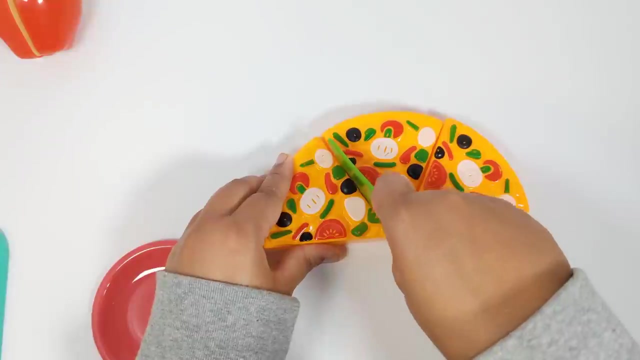 This is a pineapple. Pineapple is a yellow juicy fruit Pineapple. Here is another pizza. Pizzas are made with dough and then you add sauce and then cheese and then toppings. Toppings can be vegetables Toppings. 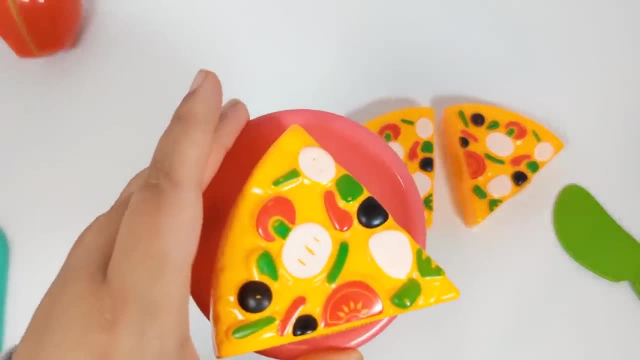 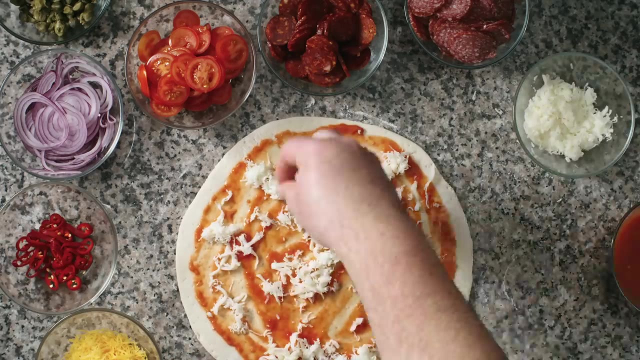 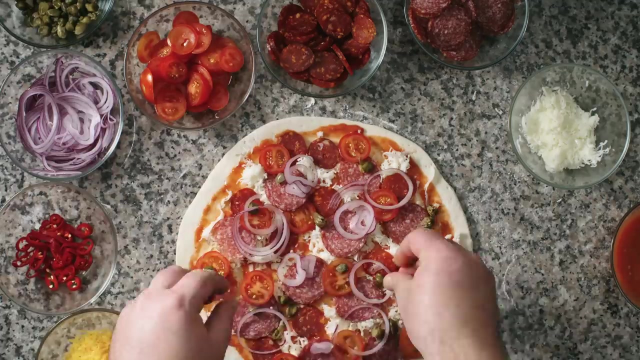 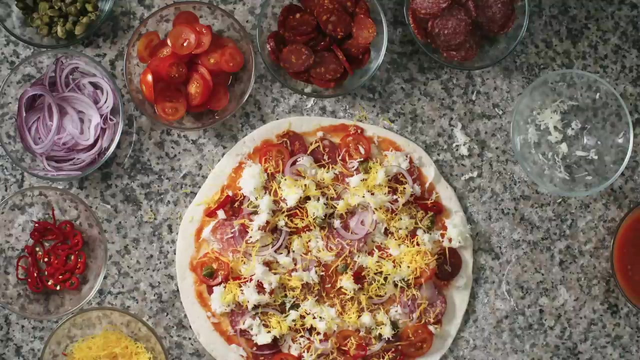 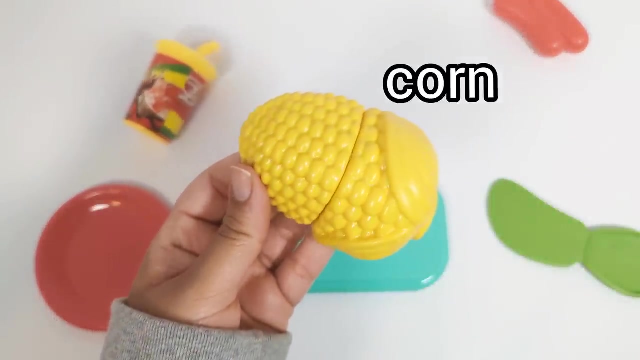 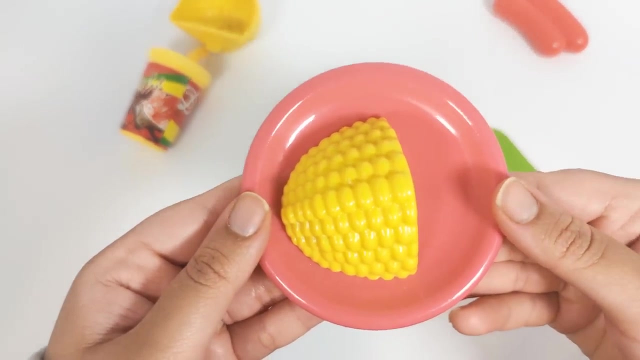 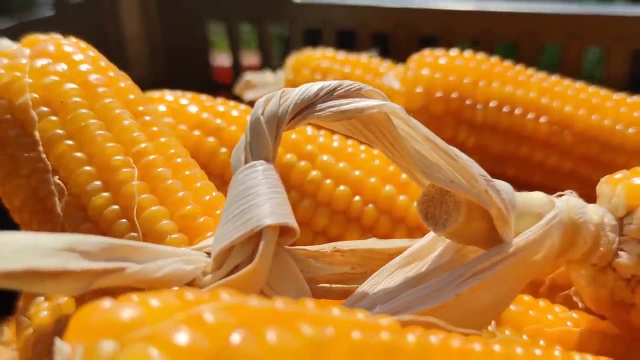 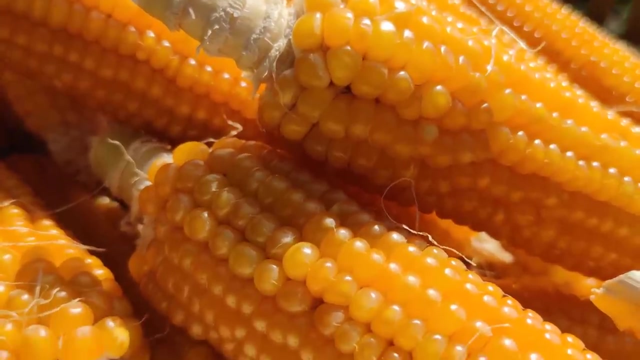 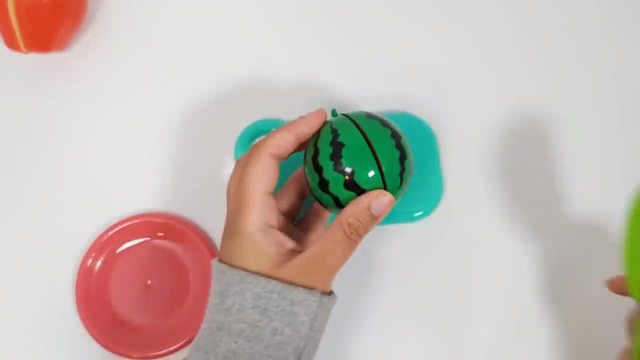 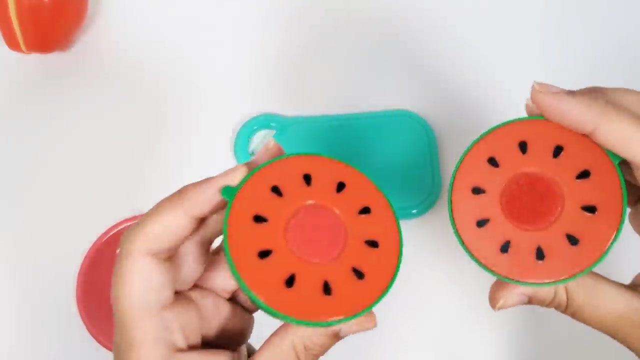 Toppings Pizza. This is corn. Corn is a vegetable Corn. This is a watermelon. A watermelon is a very delicious fruit. Wow, It was green on the outside but it's red on the inside- Watermelon.